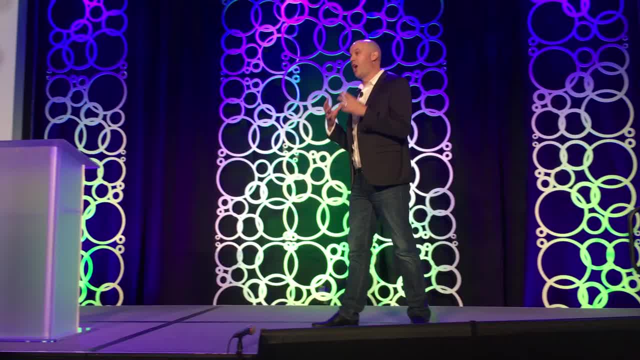 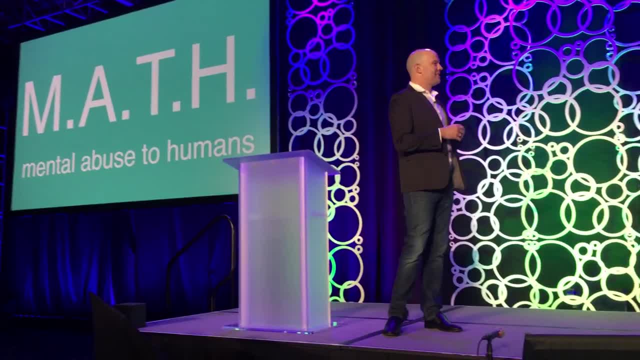 one is: what would your students say if I asked? If we're honest with ourselves, math isn't that friendly and for many of us it doesn't taste that good. We see math as a sort of grumpy uncle that I spend time with at Thanksgiving- because I'm supposed to, but I 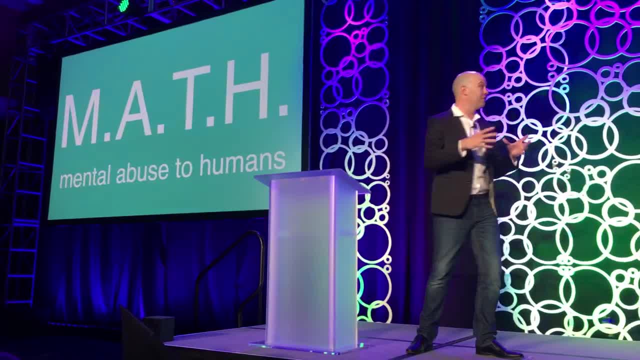 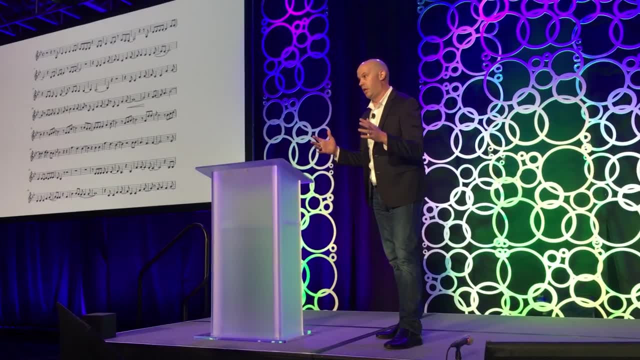 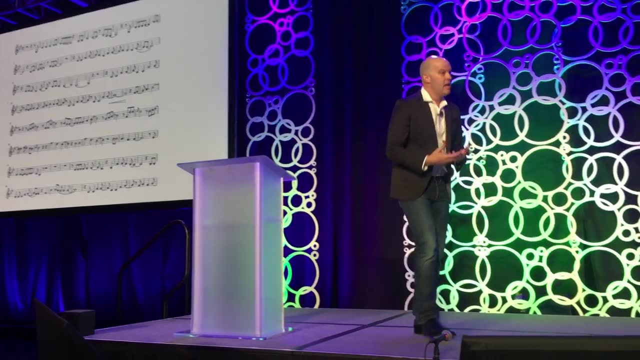 absolutely do not want to disrupt the status quo. You never know what you're going to get. If math did an analogy with music, we would say the only way to experience music is if you manipulated symbols on the page but never listen to the song. It doesn't make sense that, whether digital or not, we experience. 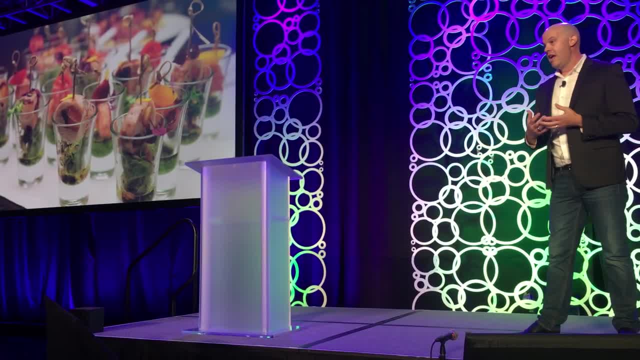 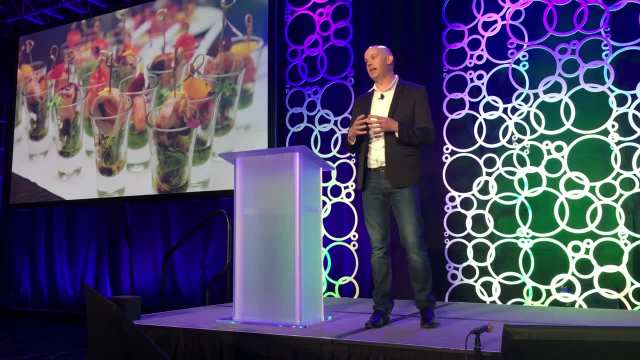 mathematics without any sort of appetizing flavor. It's just worksheets all the time. What are we really getting Imagine instead, if we pulled from this that math was appetizing and it was desirable? It's not just student achievement that we need. Research shows. 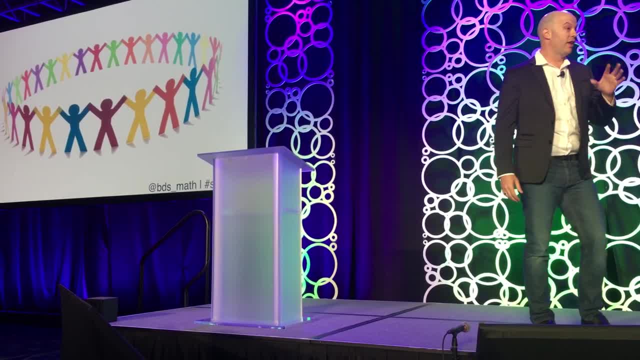 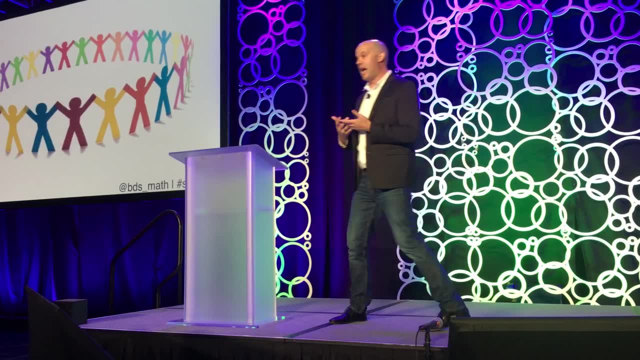 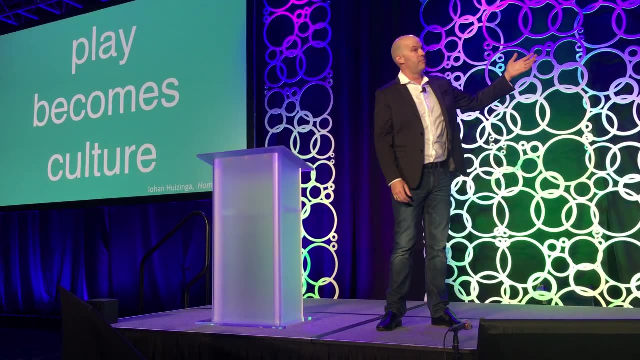 that parents math anxiety directly and negatively correlates with student achievement. We need to build a community of support around our students, but the question is: is how do you change a culture around math? The founder of modern cultural history said: play becomes culture. So we do this by setting 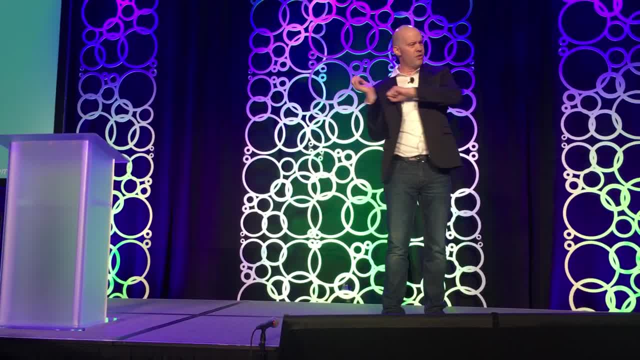 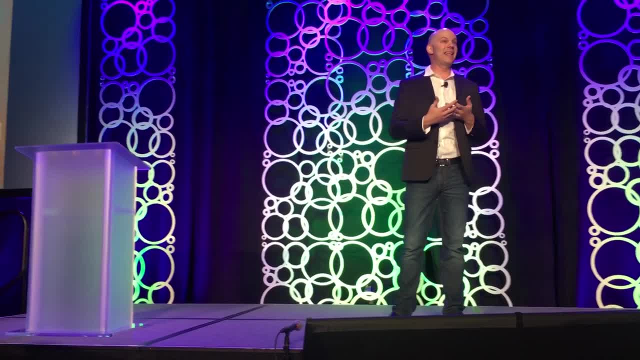 out to create great mathematical play. We throw dice out the window. There's no flashcards, You don't get a point for writing down an equation. Instead, we go to the roots of math itself In Africa. we take existing games that have already 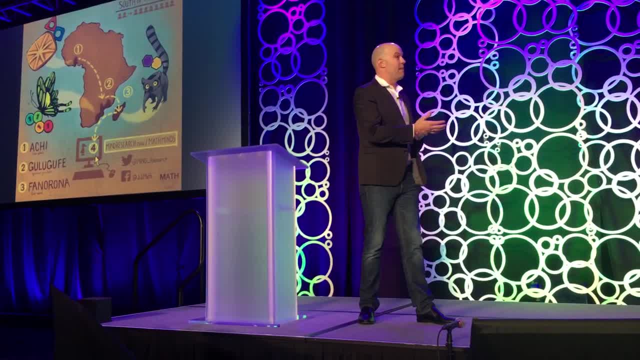 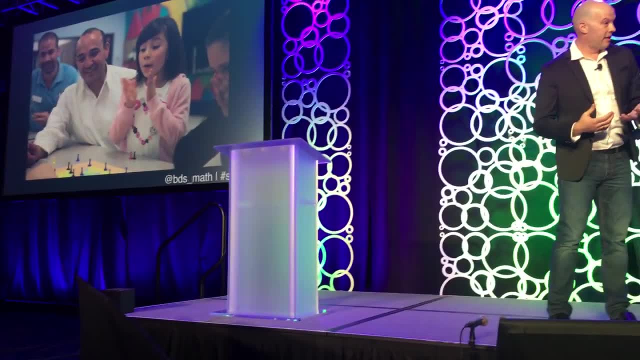 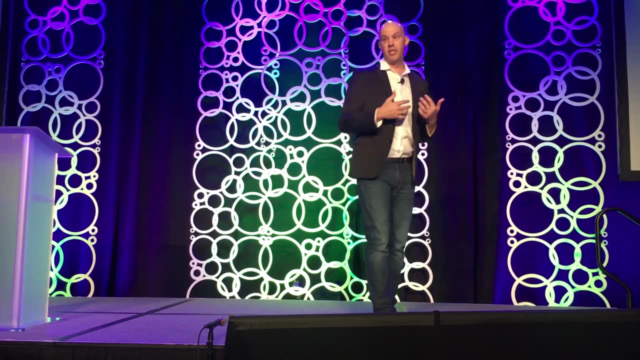 proven to be cultural powerhouses and infuse mathematics directly into the experience. You don't stop the game to do a math fact. You play math. Adults and kids play together in a meaningful way. Where adults are challenged, kids get more than just math facts. Everybody is. 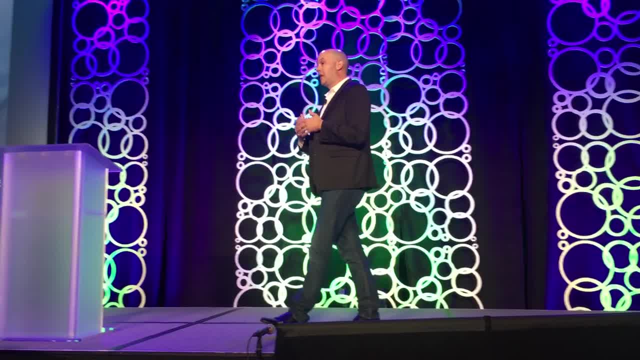 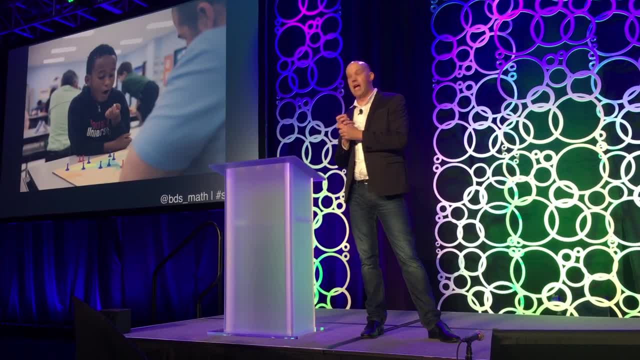 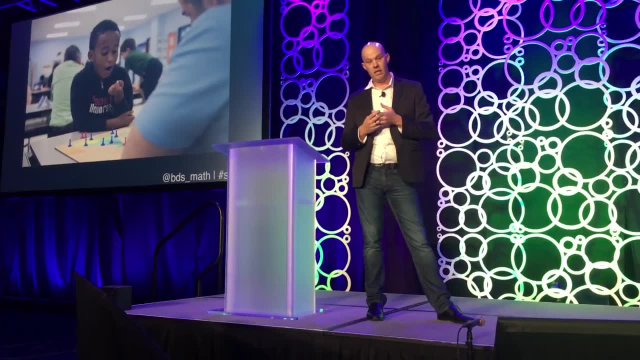 dynamically active. Not only are these games a lot more fun, they increase rigor. Too often with math games, we spend all of this time motivating you to something that I could get without the game anyway. Here we carry and compel you through deeper learning, But this highlighted a really big problem. If you 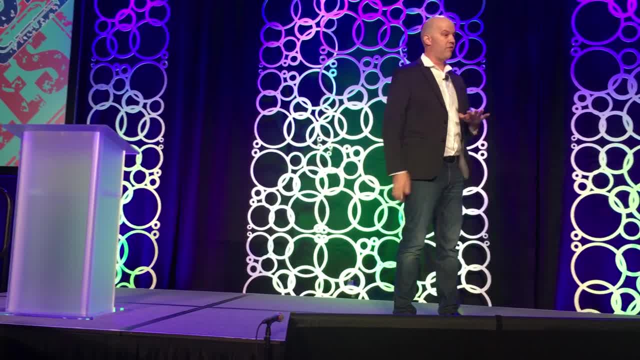 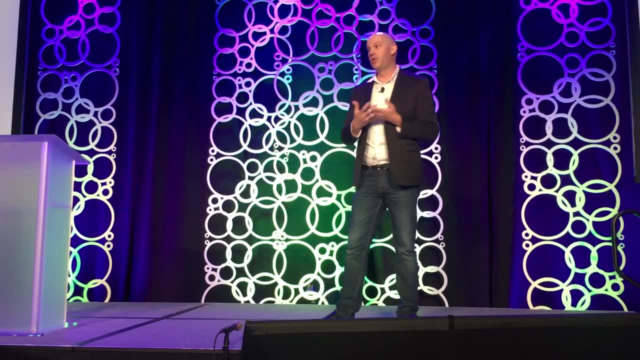 use game rules to scale a game that you've never learned before, it falls flat. Great mathematical play requires that we build great learning. We have to do something that game rules can't, and we went to stories to make that happen. But we have to be careful. We didn't want to. 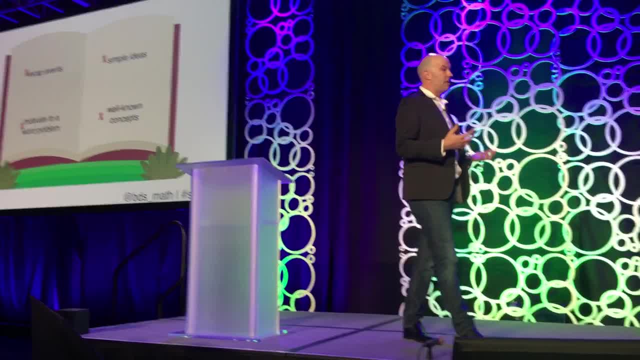 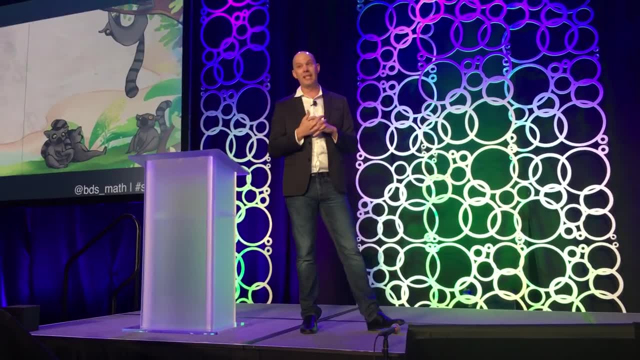 just motivate you to do a word problem or teach the simple stuff, like we see in math class all the time. We want stories to be a new technology that can build deep and conceptual understandings of complex ideas. To do that, we went back to the countries of origin. We use historical 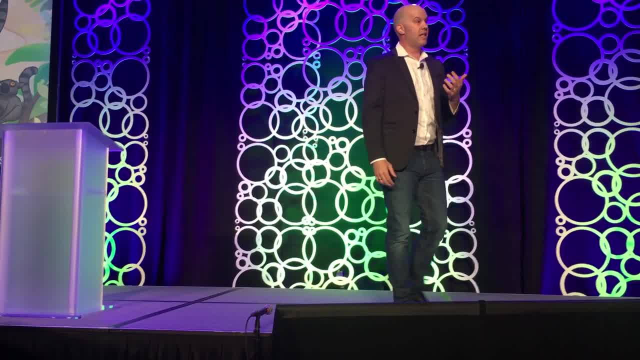 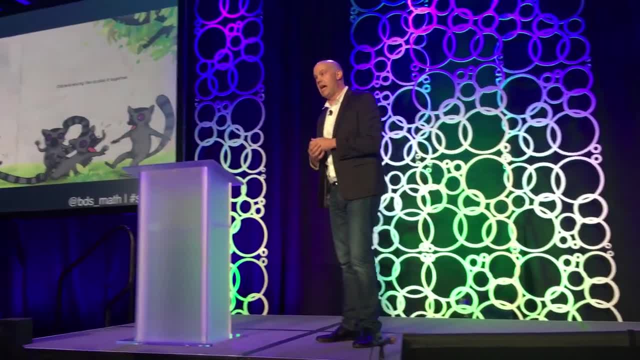 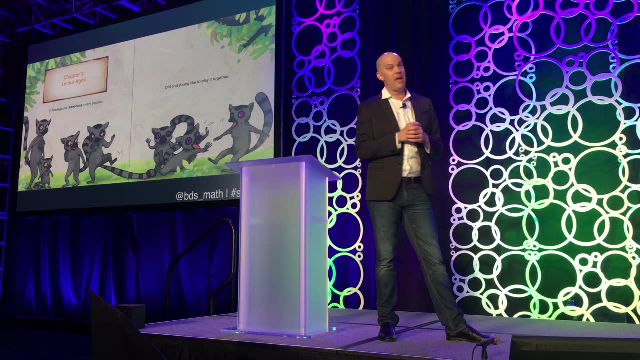 history to create real-world insights so that the learning of the game made sense and it was grounded. The real world is full of models that can ground our learning and, especially, make gameplay natural. The stories now carry us through that learning path. The gameplay is fun, it makes sense and math again becomes. 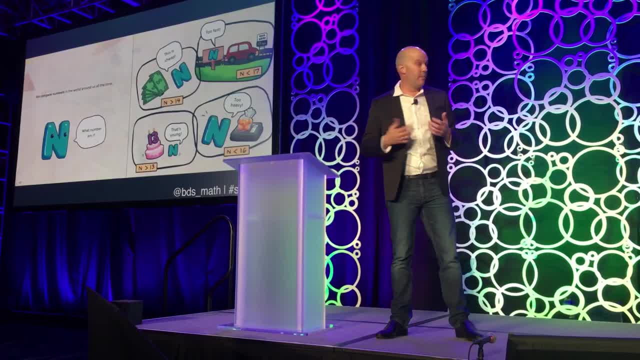 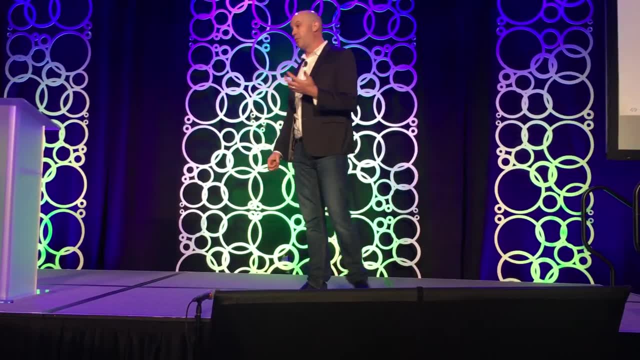 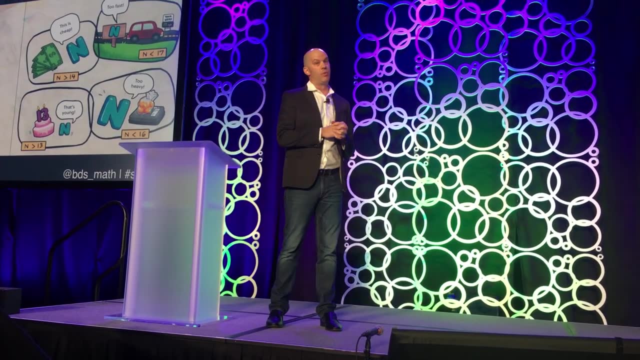 naturally infused in the progression of the story, further building that friendship with math. If stories can teach complex ideas in a global context, if games can increase rigor and math invigorates all this, it sounds great but doesn't actually work. Our story is better than game rules. We tested this with 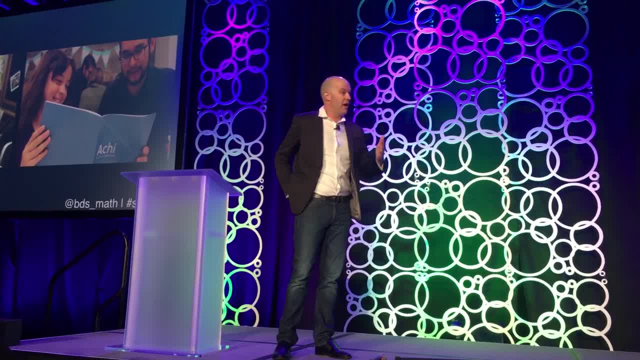 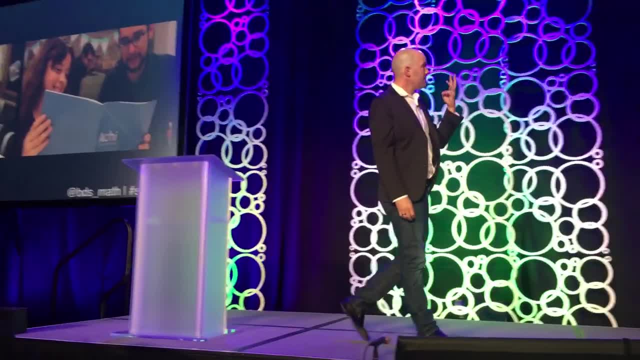 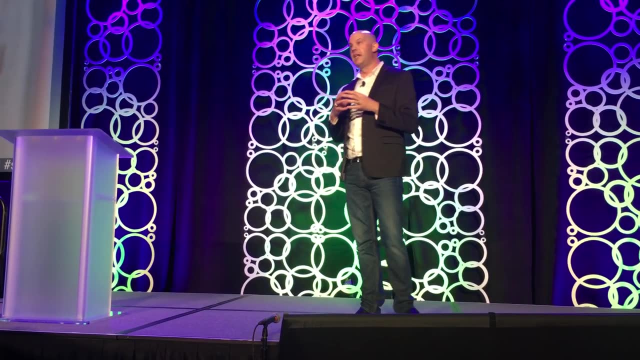 over a thousand people and found that, across the board, parents and kids can and will learn the games. They'll stick with the games longer, they'll play the games correctly and they exhibit a much deeper level of critical and mathematical thinking. If we can allow ourselves to fundamentally reimagine how we work with 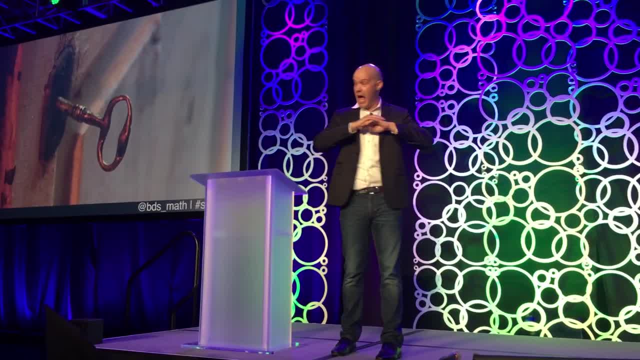 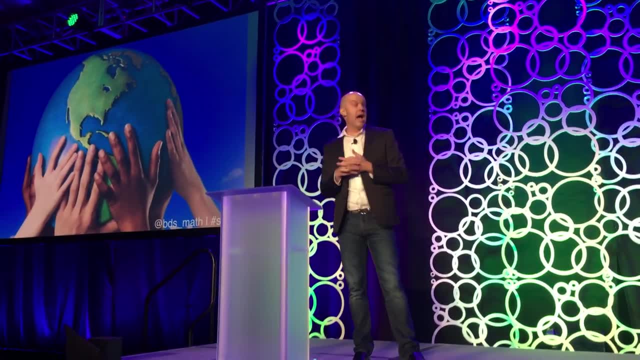 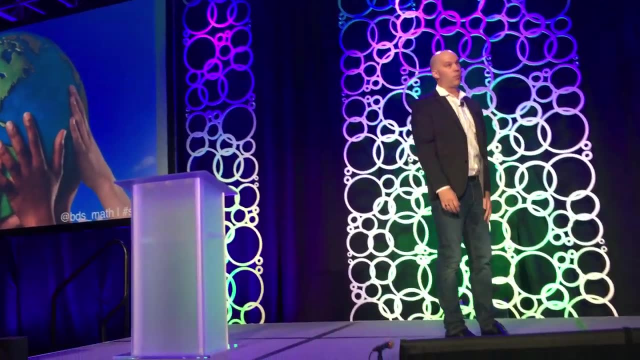 mathematics, We unlock the door for every human experience to become a mathematical one. Imagine if our students, as they go into the world, had a friend by their side: mathematics. They chose to use it and they knew it well. They could solve the world's most challenging problems. 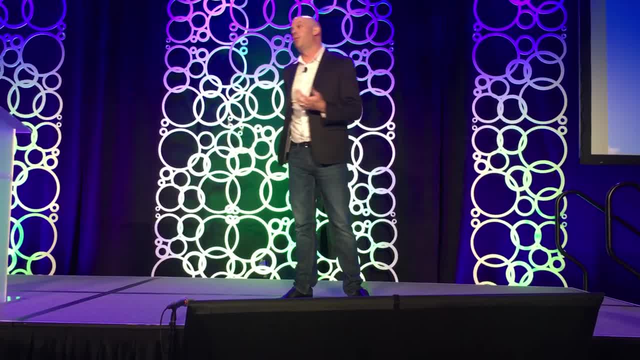 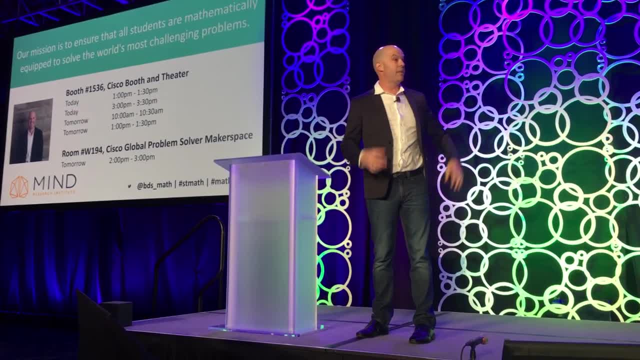 That is our mission at Mind Research Institute. If you would like to hear more about who we are as a social benefit organization, please follow us on Twitter And tomorrow at 2 pm we are going to do a sneak peek product reveal of what these games and stories look like and you will be able. 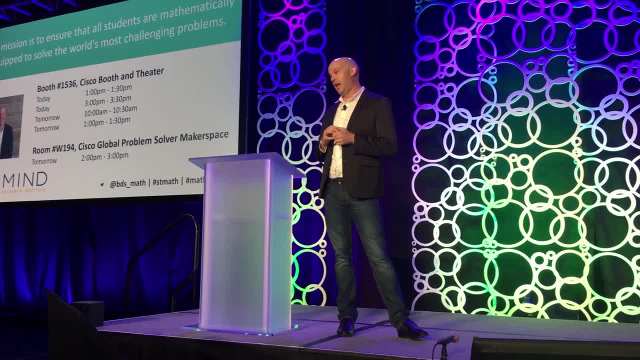 to experience firsthand guided mathematical play through story. Enjoy your conference, Thank you.